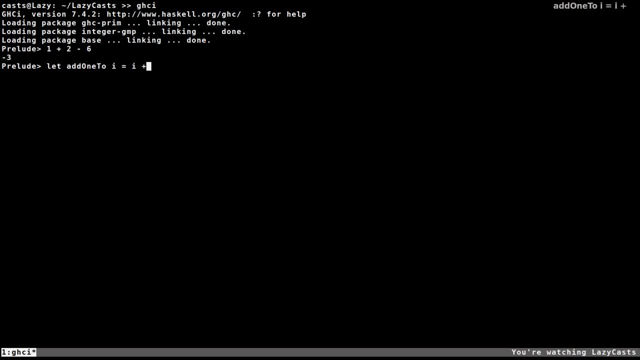 First write let then the function name and then define the argument, which is the number you want to add one to. Then we can just write the argument plus one. So if we want to try this out, we just type out the function with a number and we get the result. 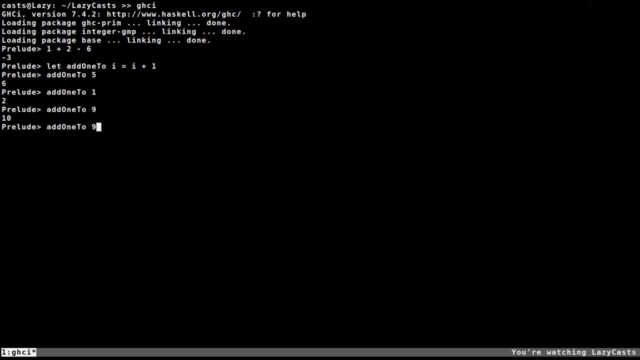 We can try it with any number we want. We'll always get the correct result. GHCI is great. However, when we restart GHCI, everything is lost and we need to rewrite everything again. So instead, let's write our functions inside a file and load it into GHCI. 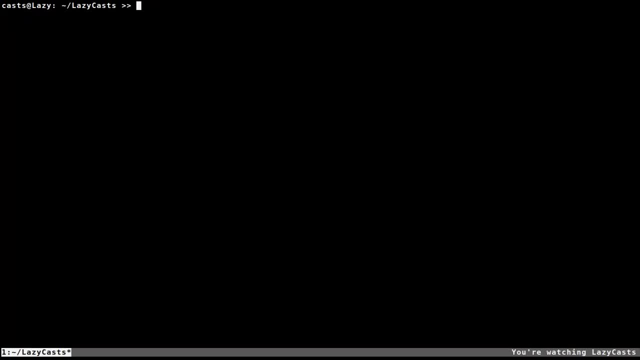 We'll call this file mainhs. Now, writing functions is slightly different here. We don't need to write them with let. to begin with, Let's rewrite our previous function. GHCI is the same. The function is the same, except only if we write a function with let. 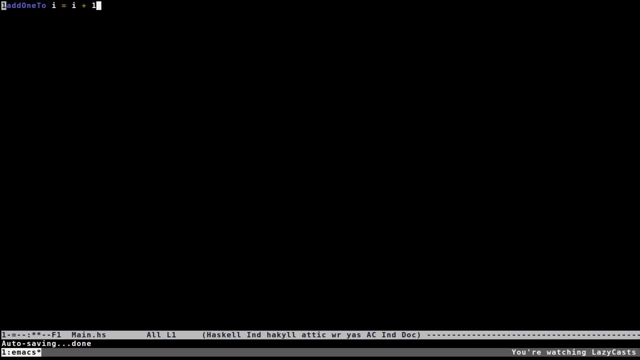 As you can see, it's the same, except we're not running let. here We only need to write let. We want to write nested functions. Here's an example: Let's write a function that takes two numbers and outputs two numbers. However, if either one of the numbers are not even, we extract one from that number to make it even. 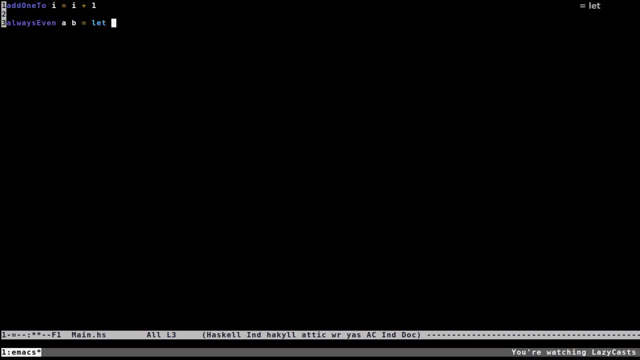 GHCI is the same. GHCI is the same. GHCI is the same. Here we define a function that takes two arguments, a and b. Inside of this function, we define a nested function as a let expression isEven. isEven takes one argument and then does an. 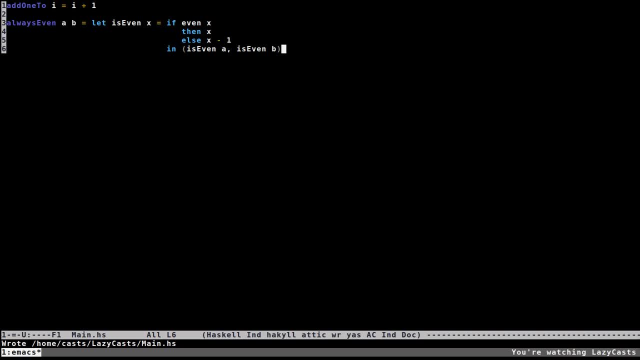 if statement checking if the number is, even with the even function, Even x, returns a boolean, in which you guessed it: if x is even, it returns true, if it is uneven, it returns false. So, if x is even, we get x, if it is uneven, we get x-1, which makes it even Once you're. 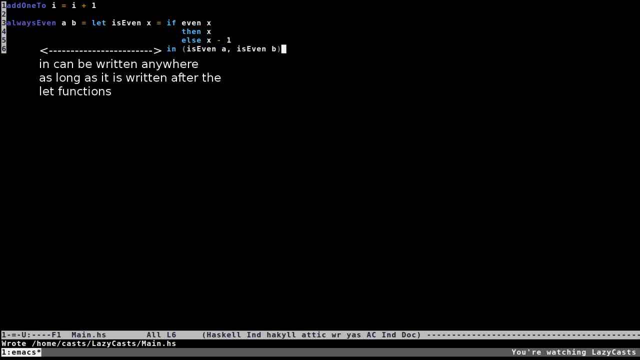 done writing your let functions you have to write in. so we know we're done writing nested functions After in. we say that the output value of the always even function is a and b. However, we supply those values with the isEven function. This way we don't have 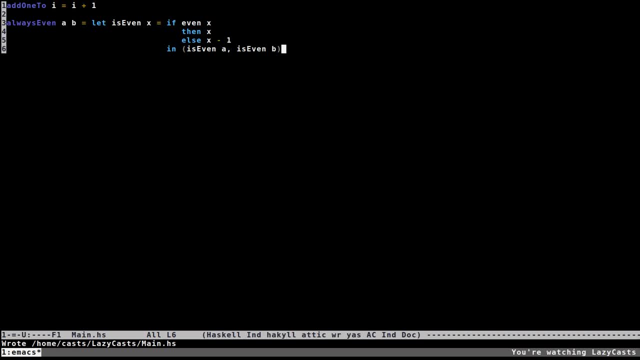 to write the if statement twice. Not only that, isEven cannot be accurate. Don't worry about the parentheses right now. I'll be explaining those in the next episode. Let's test this function out in GHCI. To load files into GHCI, you need to open GHCI in the same directory as the file and 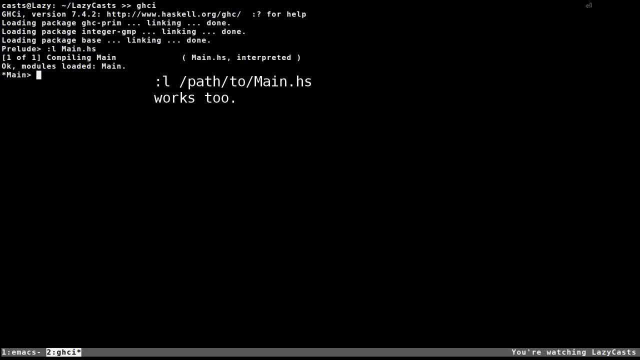 type colon l and the file name. The l stands for load. If all went well, the file should be loaded correctly. If you get an error message, then you might have written the function wrong. Let's test the function out. It works. Now we can write our code inside of a file and test it in GHCI. 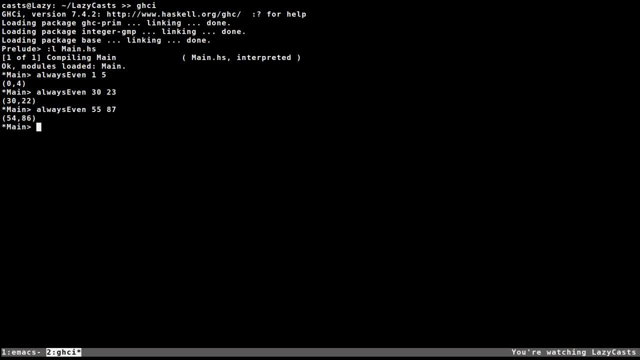 Also note we can't call the nested function isEven. If we try, we'll get an out of scope error. This is helpful because we can pollute the rest of our code with isEven. If we try to call it in our program anywhere else, we'll get an error at compile time, which saves. 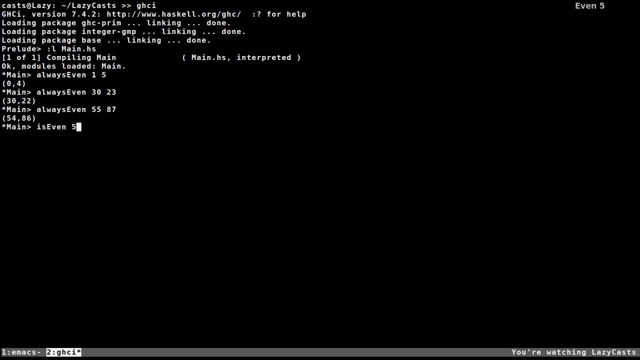 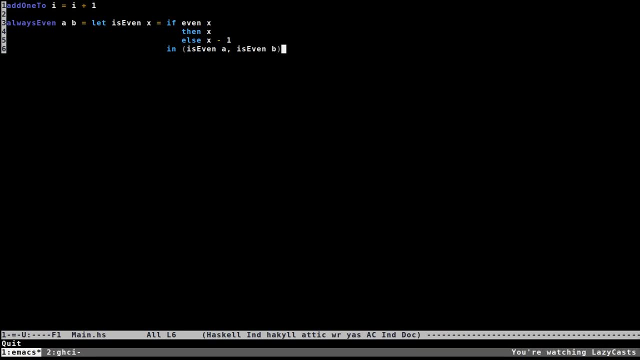 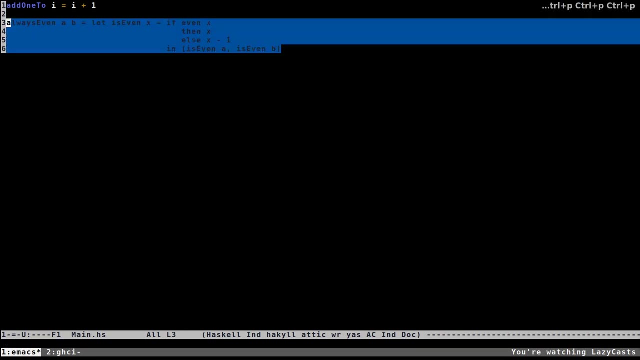 debugging. There's another way we can write nested functions in Haskell. That is by using where instead of let. Let's adjust this function for that. As you can see, we can write nested functions in Haskell by using where instead of let Let's adjust this function for that. As you can see, we can write nested functions in Haskell by using where instead of let. AS you can see, we can write nested functions in Haskell by using where instead of let. As you can see, we can write nested functions in Haskell by using where instead of let. 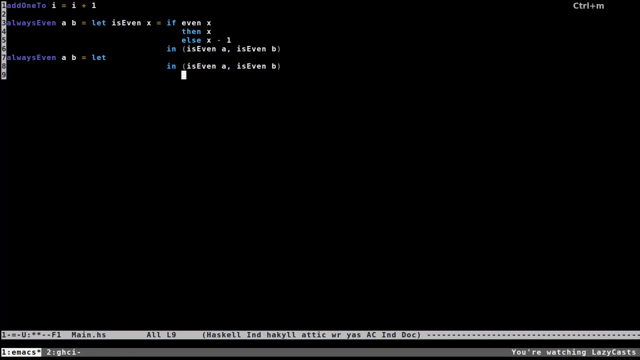 Let's check it on our script Now. bear with me here because it might look a bit confusing at first. Why can't be use isEven, even though it's written in after it's called Everything written inside of where can be used anywhere inside of the parent function? 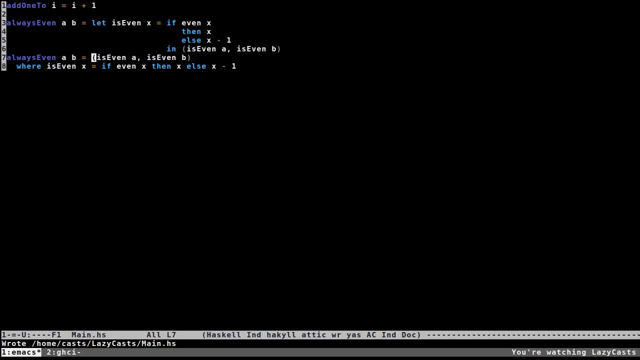 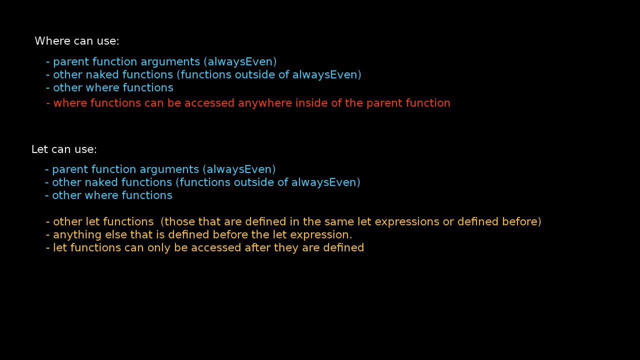 so it doesn't matter if it's written after it's called, unlike the let expression. This works almost the same as let, but with a few key differences, Where- and let. both have access to the parent function's arguments. other naked functions. 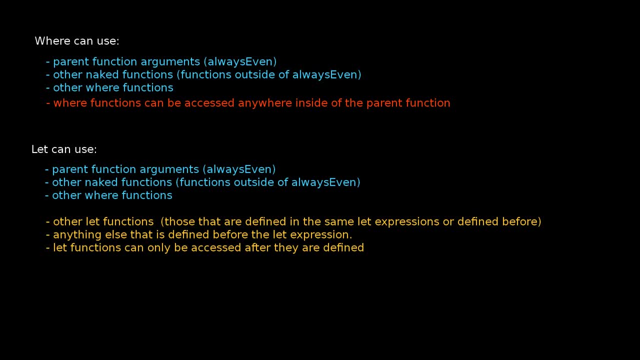 and other where functions. Let, however, can also access anything that is defined before itself. So if a value is defined inside of the parent function, where cannot access it, but let could if it is defined afterwards. So, as you can see, let has more access to other values than where. so it's completely. 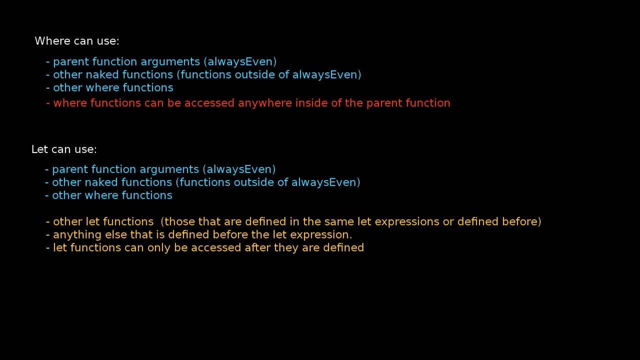 situational as to when you will want to use where or let. I personally find where a bit more clearer, so I try to use that as much as possible. However, in some situations you have to use let. Before I continue my explanation on function, let I want to mention that there are some. 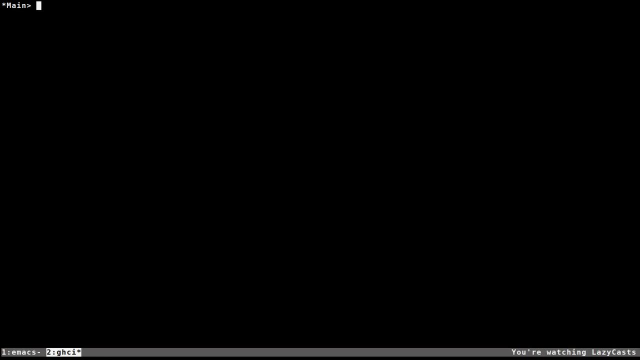 other ways to use let, For example, if you want to check if something is not equal to something else. I would like to talk about equality checks really quick. A lot of people that start learning Haskell trip over this simple thing. Basically, if you want to check if something is not equal to something else, you have to. 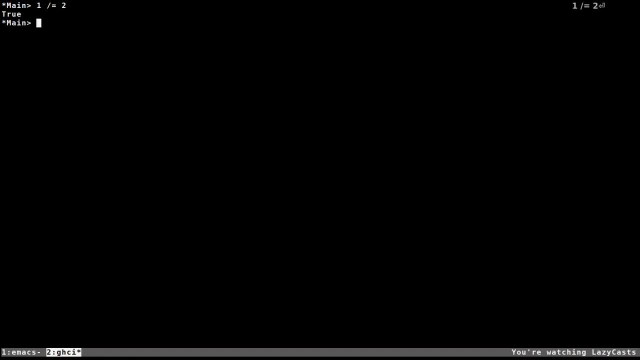 write it like this. In almost any other language, it would be this Which is incorrect. However, if you want to check if something is the same as something else, it is the same as almost any other language. Let's talk a bit about functions. 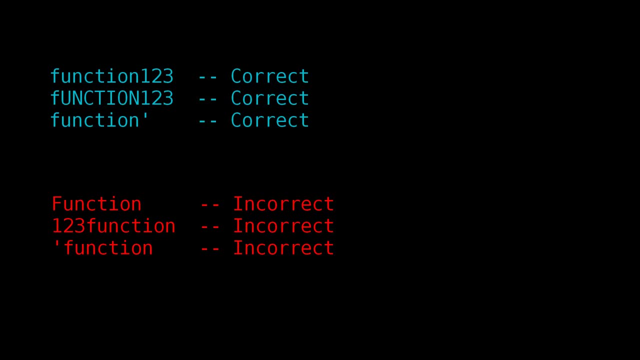 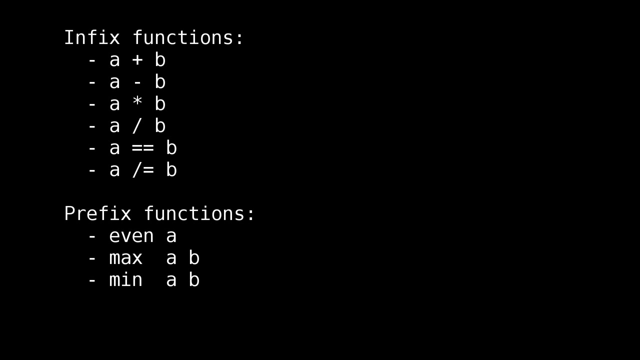 Make sure that the first character of a function is always a lowercase letter. A function can contain letters, numbers and single quotes. This applies to arguments as well. Plus, minus and slash are also functions. however, they are called infix functions. 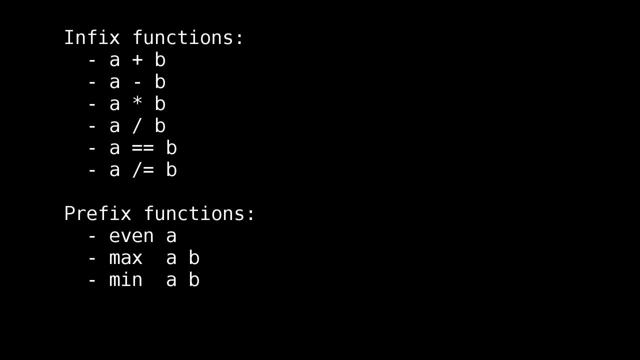 They are functions that take an argument on the left and an argument on the right, instead of having two arguments on the right. Let's talk a bit about functions. We can also write our own infix function. they can be made out of a lot of different.